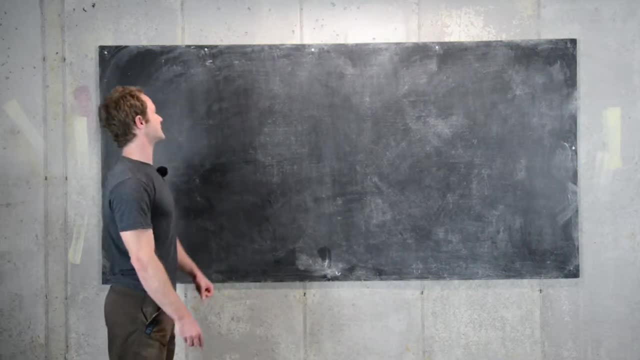 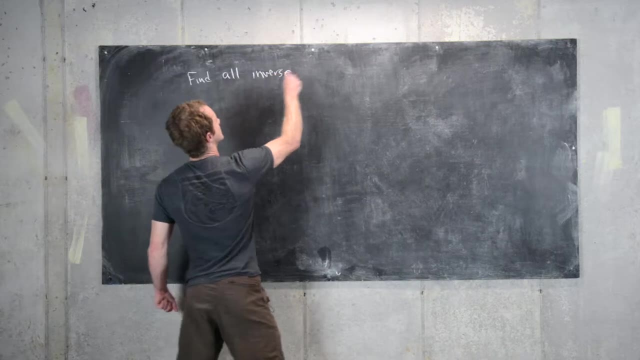 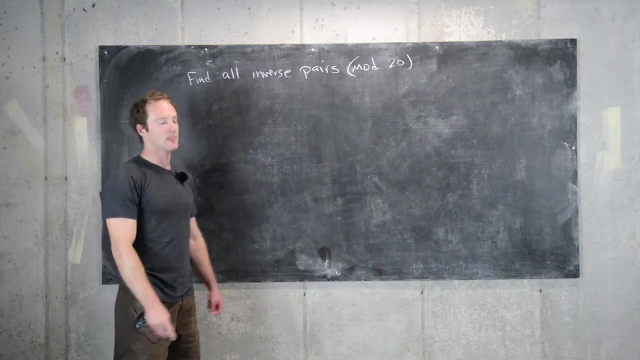 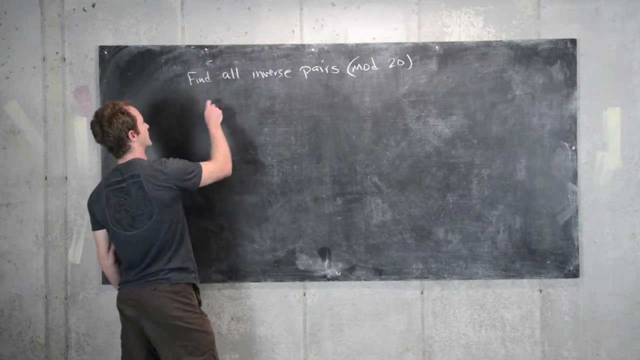 Okay, good. So let's start with the one that is small. So let's find all inverse pairs: mod 20.. Okay, great. So again from a previous video, we know that the invertible numbers mod 20 are the following: 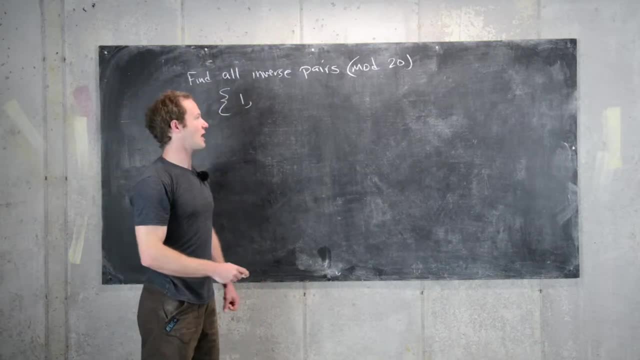 So we have 1.. So it's going to be everything that's relatively primed to 20.. So 20 has prime factors 2 and 5, so it should be fairly easy to write down a list. So we have 1, 3.. So we can't have 5, because that's a multiple of 20.. 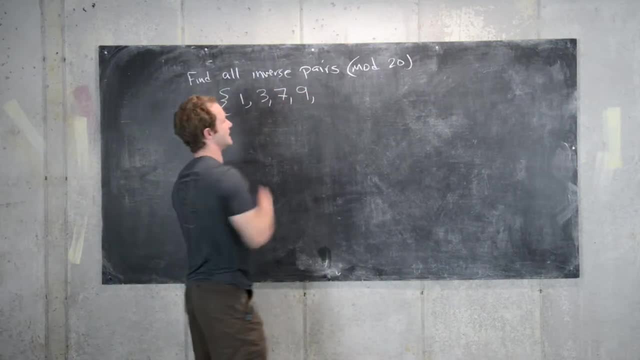 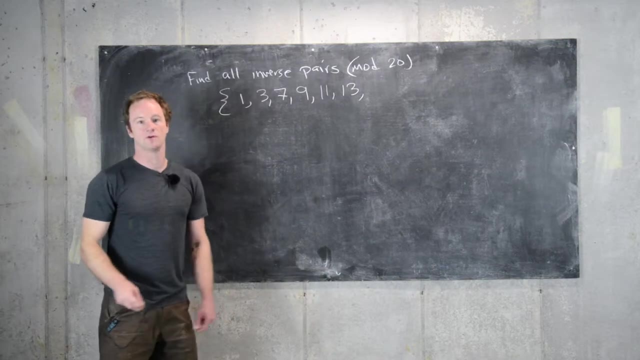 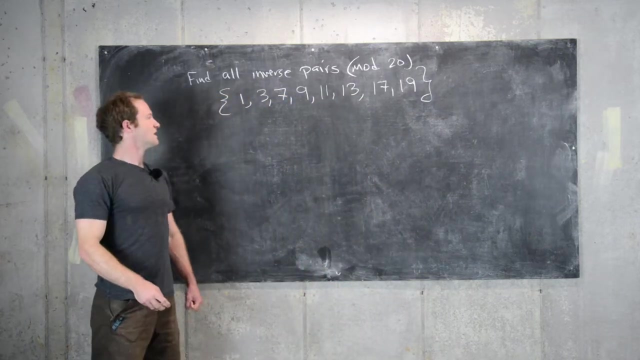 So 7 is next, 9 is next- So notice I'm skipping all the even numbers. 11 is next, 13 is. after that We skip 15,, 17, and 19.. So now let's get started with the kind of easy ones. 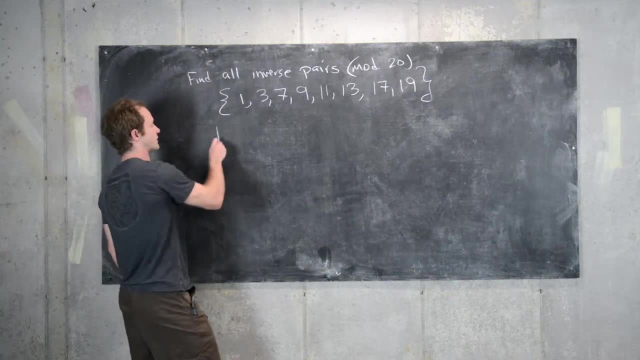 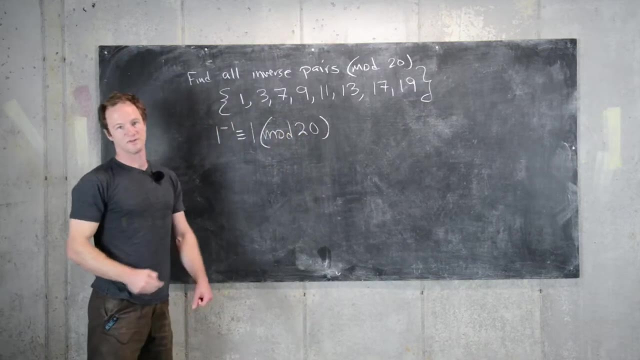 So notice: 1 is its own inverse, So we can write that down: 1 inverse is congruent to 1 mod 20.. That will always be the case Now we work up from there. So 3 times 7 is 21.. 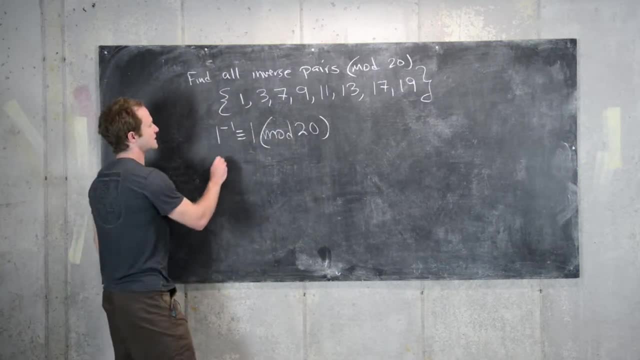 And so 21 is 1 mod 20, so that's lucky. So 3 inverse is congruent to 7 mod 20.. So 3 inverse is congruent to 7 mod 20.. So 3 inverse is congruent to 7 mod 20.. 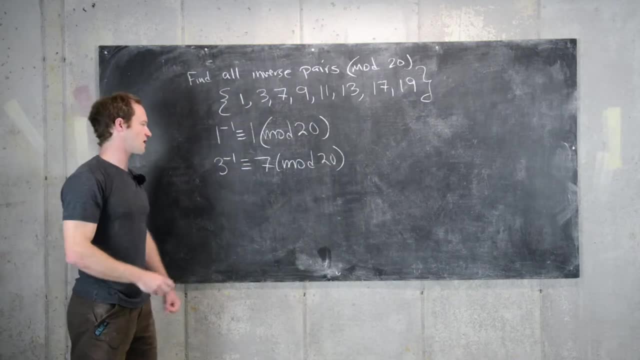 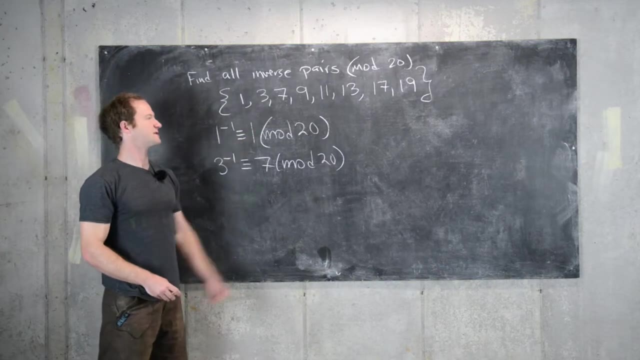 And likewise 7 inverse is congruent to 3 mod 20.. So we won't write that down, but this inverse relationship is mutual. Now let's move up to 9.. So 9 times 9 is 81,, which is 1 more than a multiple of 20.. 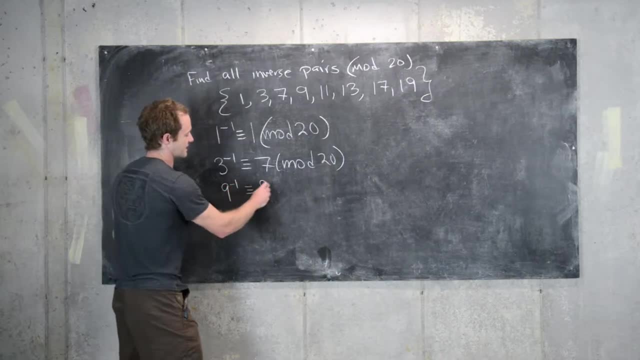 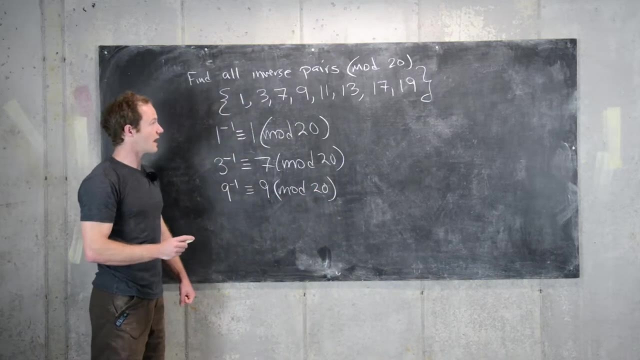 So we have 9. inverse is congruent to 9 mod 20.. So 9 is its own inverse, Great. And now we get into the numbers that are alike. These are the numbers that are a little bit bigger and might be a bit trickier to figure out. 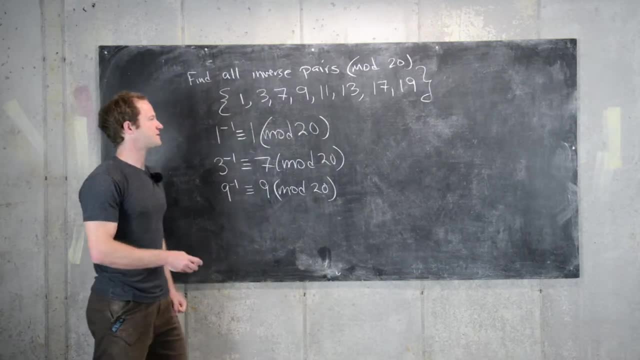 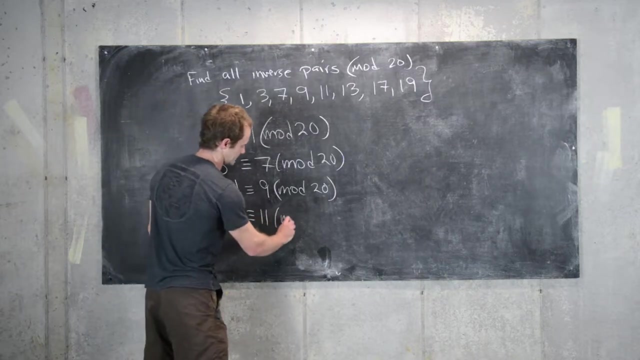 So let's go to 11.. So 11 times 11 is 121.. Oh, but luckily 121 is 1 more than a multiple of 20.. So that means 11 inverse is congruent to 11 mod 20.. 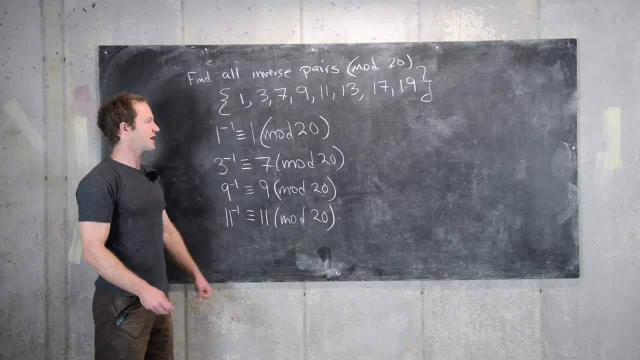 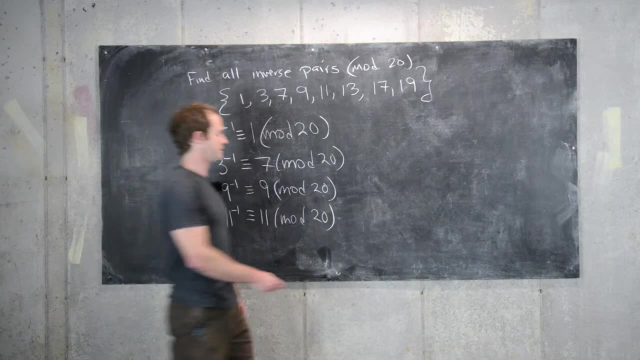 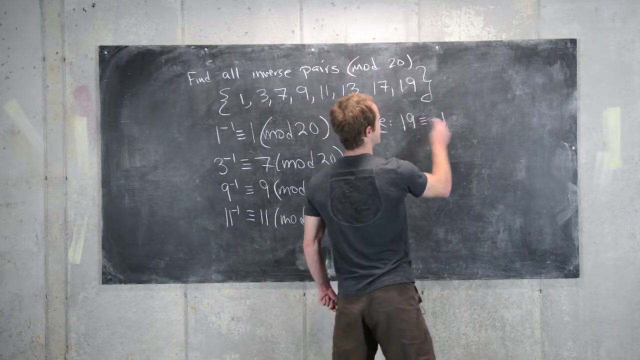 Okay, fantastic. Now we're going to use a trick for 13,, 17, and 19.. And we'll start with 19,, even though that's the largest number. So what we'll do is we'll notice that 19 is congruent to negative 1 mod 20,. 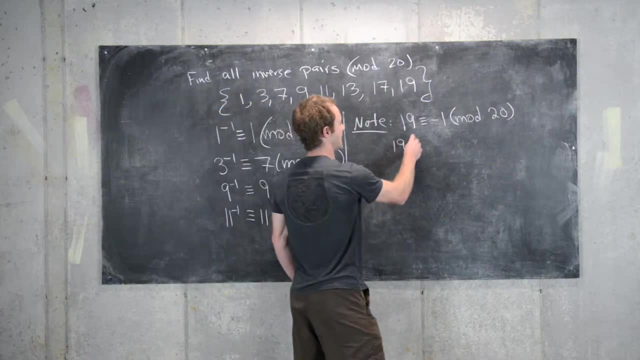 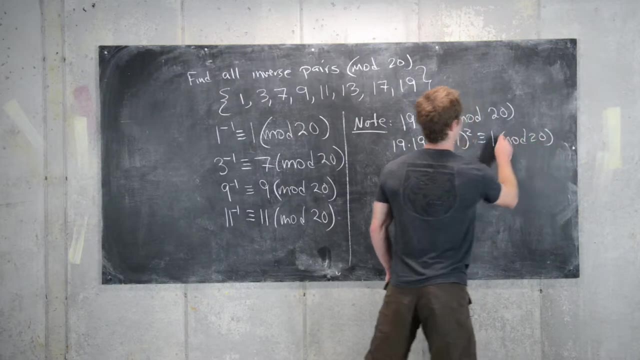 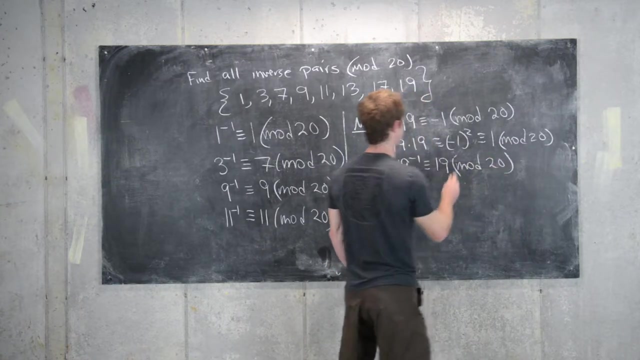 which tells us that 19 times 19 is congruent to negative 1 squared, which is congruent to 1. Mod 20.. So that means 19 inverse is congruent to 19 mod 20.. So we'll work with the negative numbers. 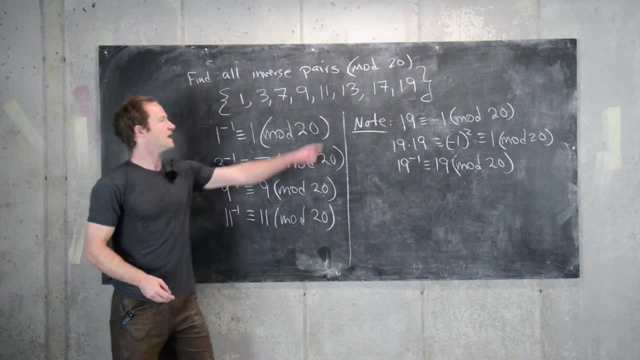 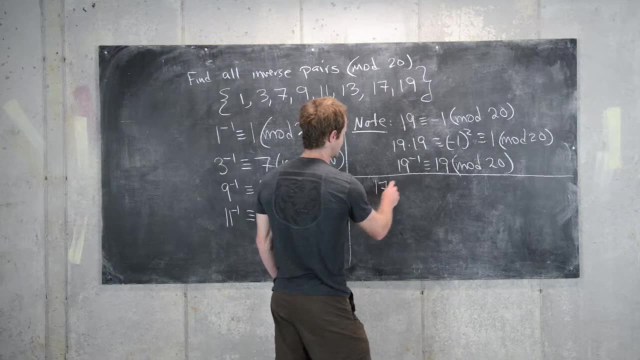 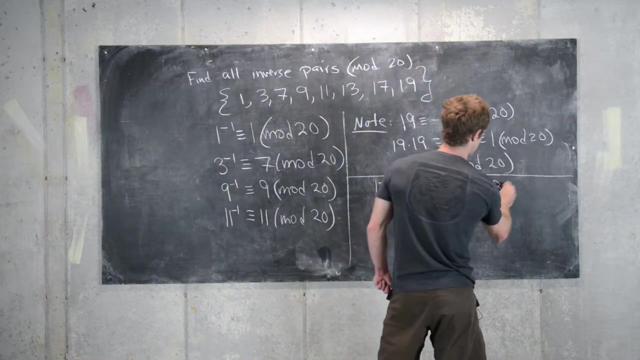 And it makes it a little bit easier because we can work with smaller negative numbers. Now we'll do the same thing for 13 and 17.. So notice that 17 is congruent to negative 3 mod 20.. 13 is congruent to negative 7 mod 20.. 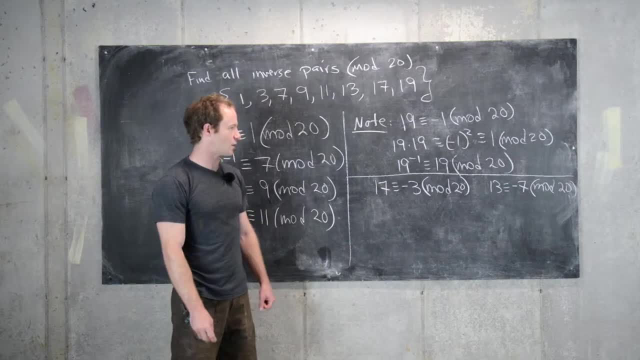 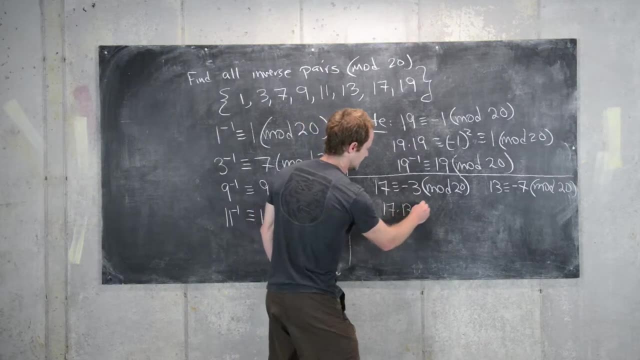 Now, when we multiply negative 3 and negative 7, we get a positive 21,, which is congruent to 1 mod 20.. So let's write that down. So 17 times 13 is congruent to negative 3 times negative 7,, which is 21,. 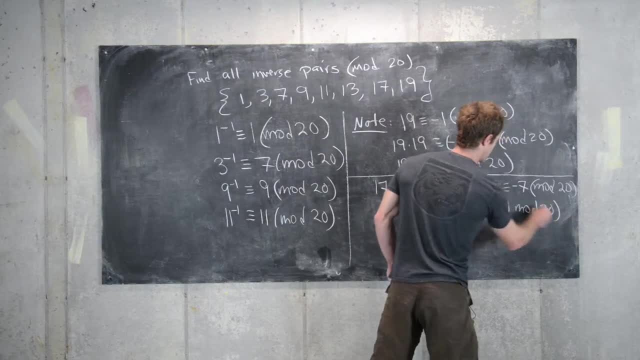 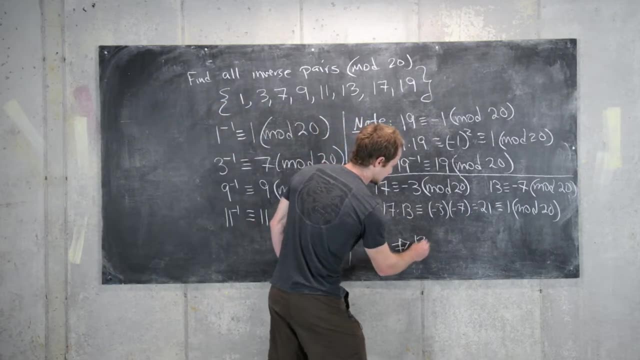 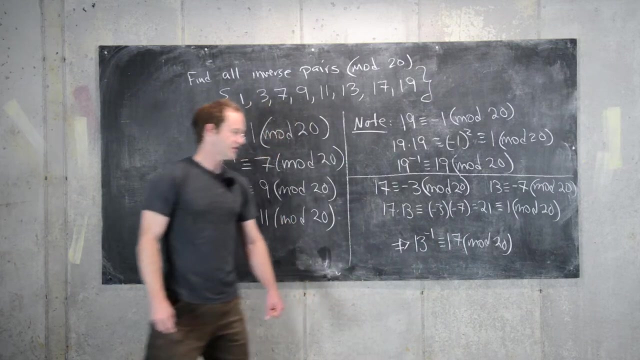 which is 1 mod 20.. Good, And finally, what that tells us is that 13, inverse, is congruent to 17 mod 20.. So, in other words, 13 and 17 are inverse pairs, mod 20.. Okay, good. 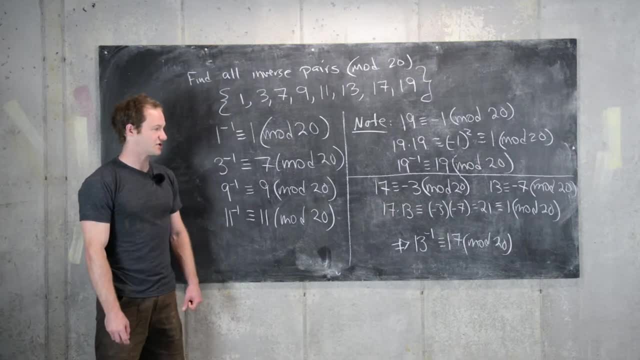 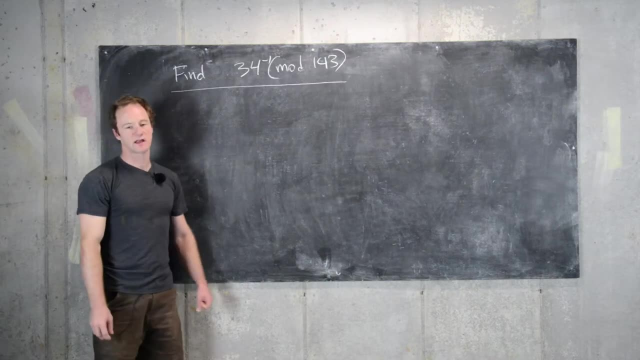 So with a number like 20, it's not so hard to guess and check the inverses. So let's look at another example where we have to do a little more calculation. Okay, so now we want to look at this slightly more difficult problem. 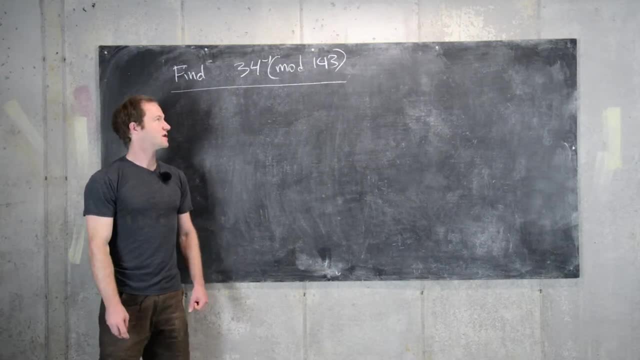 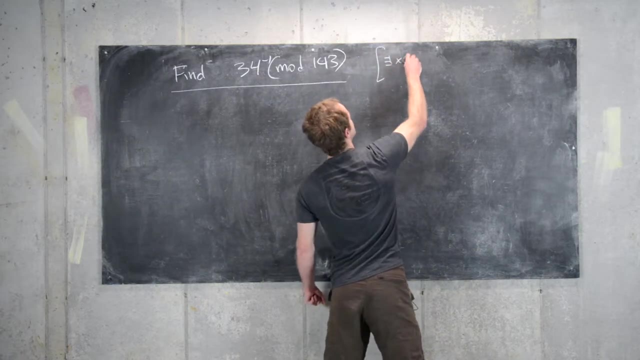 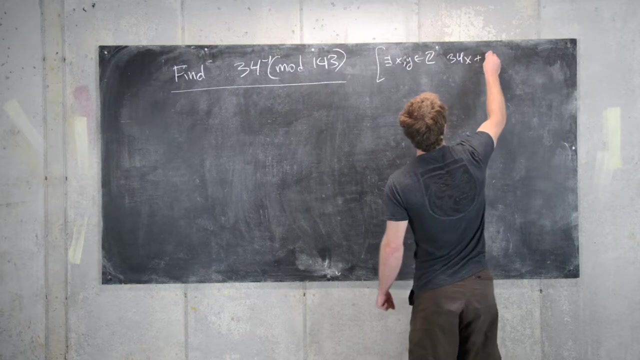 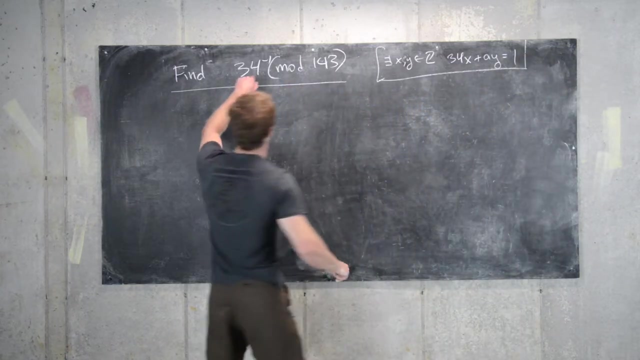 which is finding 34 inverses 34 inverse mod 143.. So we're going to use the fact that there exist integers x and y such that 34x plus a times y equals 1.. And so we haven't checked here that 34 and 143 are relatively prime. 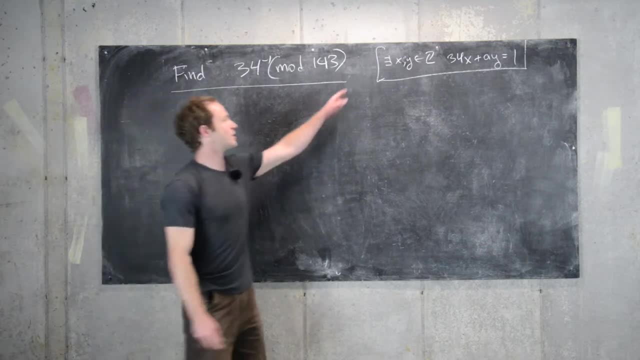 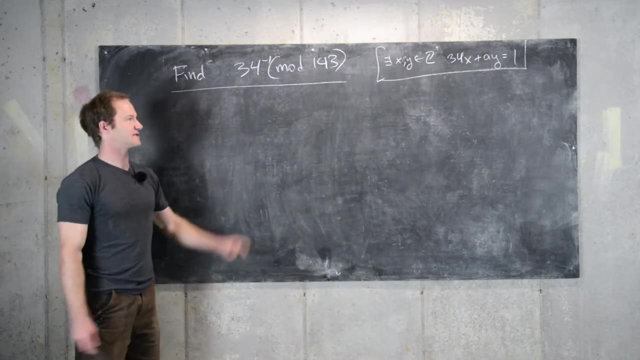 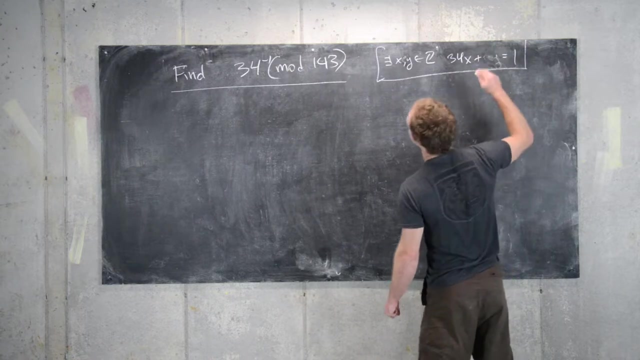 and we'll see that along the calculation, And so we'll use this fact and then we'll notice that this x value that we find will be 34 inverse, because 34 times that x value will be, and I should put here this is 143 times y. 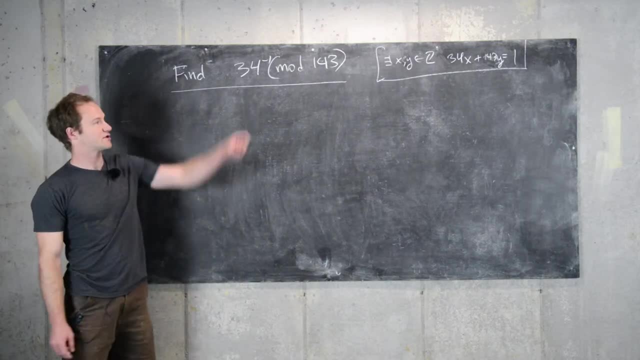 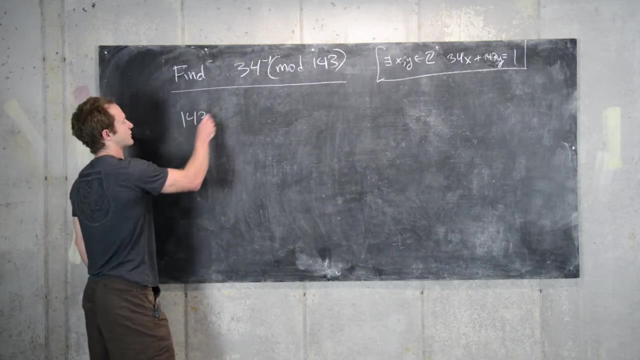 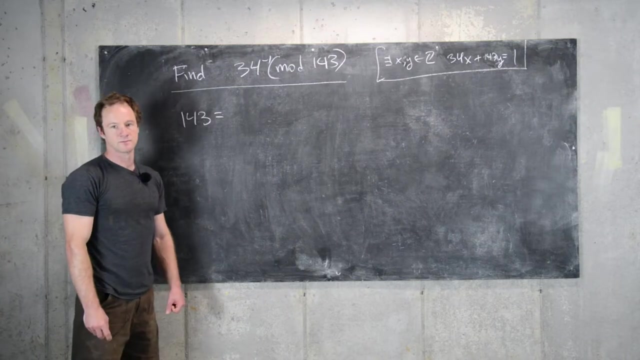 will be congruent to 1 mod 143.. Great, So since we're going for that equation, we need to use the extended Euclidean algorithm. So let's start and write 143, and the division algorithm with 34.. So there are several videos where we do this in the past. 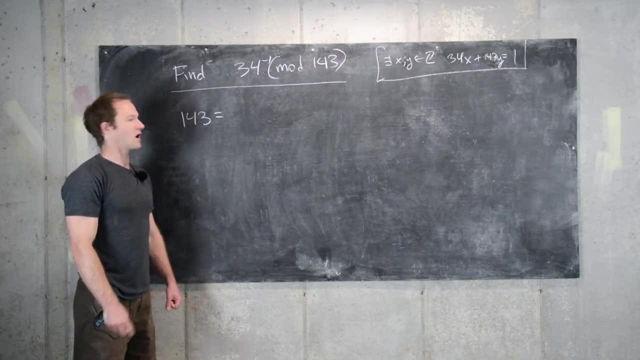 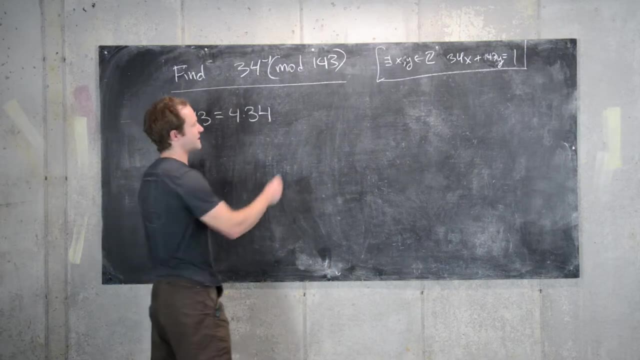 and it's a fairly routine calculation, although it can get tricky if there's a lot of steps. So this is 4 times 34 plus 7.. Good, Now we're going to take 34.. That's going to go over here. 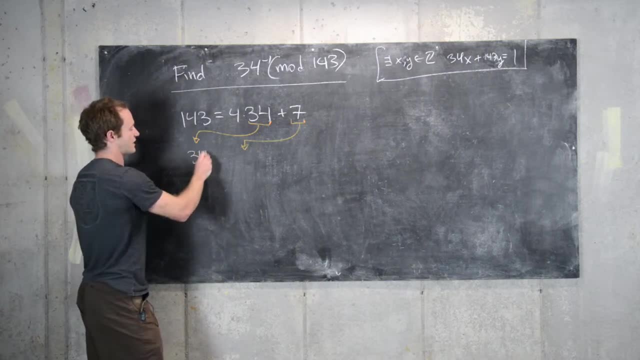 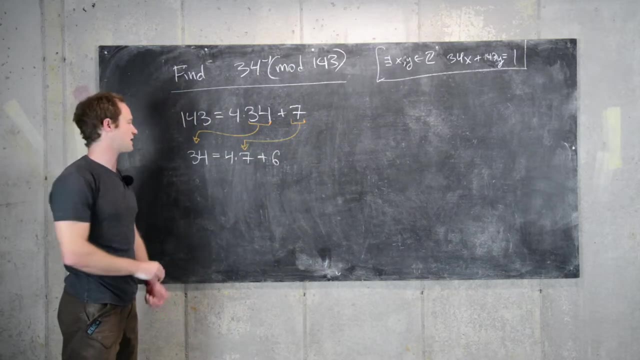 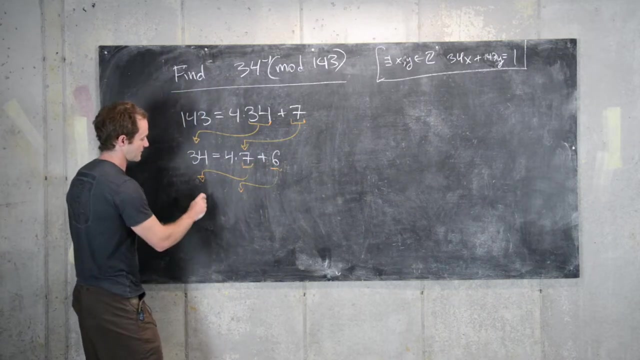 We're going to take 7.. That's going to go over here. We can write 34 as 4 times 7 plus 6.. Okay, good, Then our 7 is going to go over here and our 6 is going to go over here. 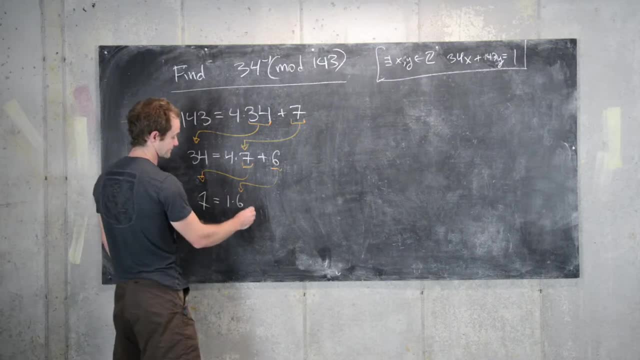 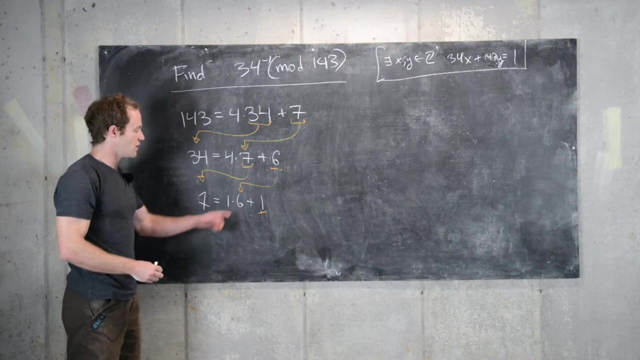 We can write 7 as 1 times 6 plus 1.. And so there we go, We get 1.. Obviously, 1 is going to be the last non-zero remainder, which tells us that 1 is the GCD of these two. 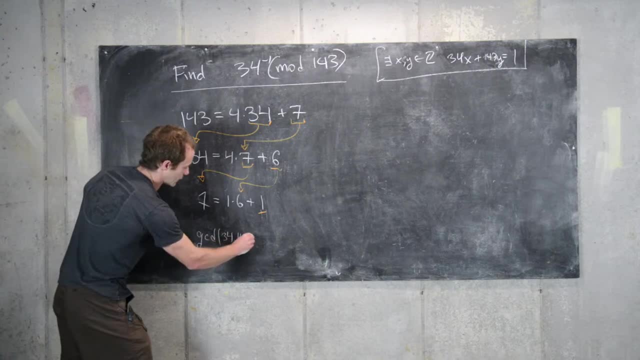 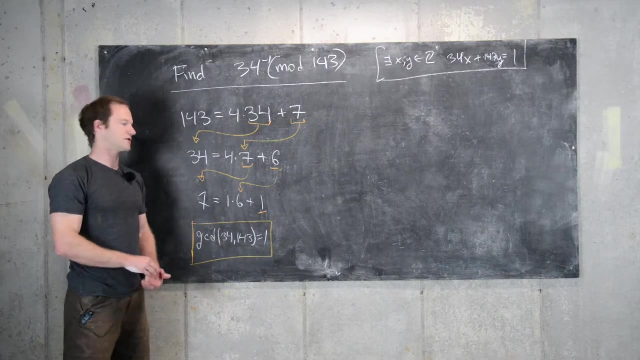 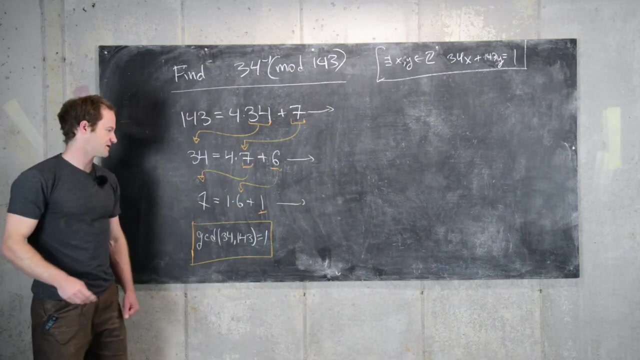 In other words, the GCD of 34 and 143 equals 1.. These numbers are relatively prime, which is a requirement for such an inverse to exist. Okay, great, So the next thing we do is we rewrite these equations, So we're going to solve for the remainders. 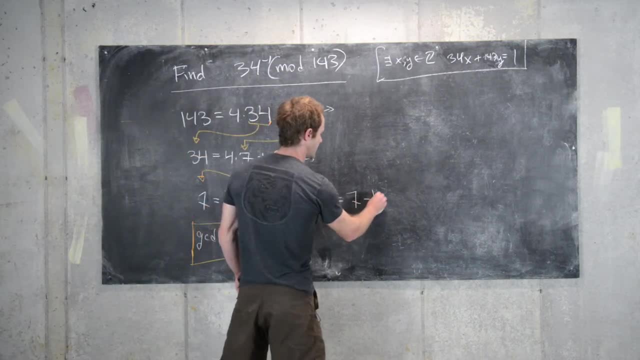 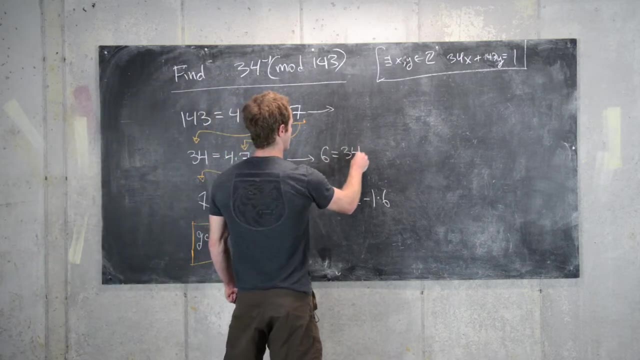 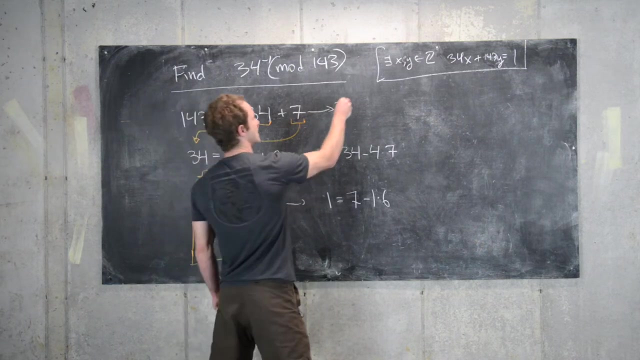 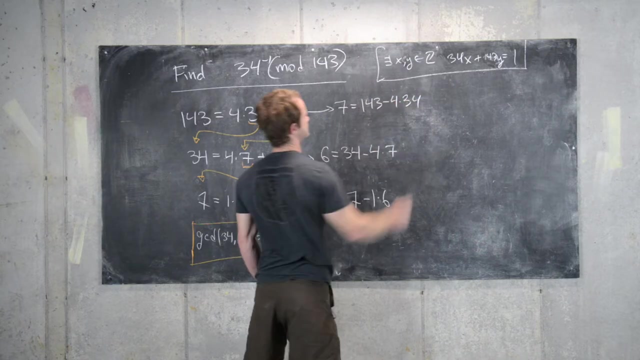 So here we'll get 1 equals 7 minus 1 times 6.. Good. And then here we'll get 6 equals 34 minus 4 times 7.. Okay, good. And then finally, here we'll get 7 equals 143 minus 4 times 34.. 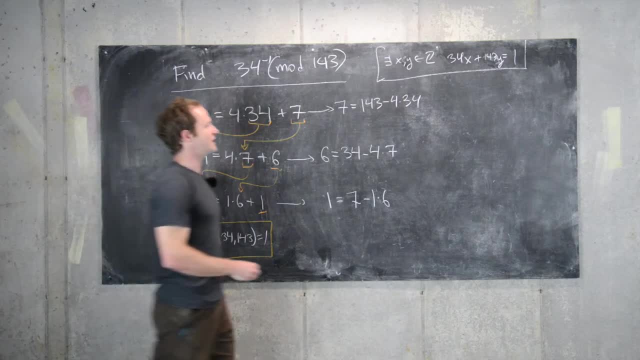 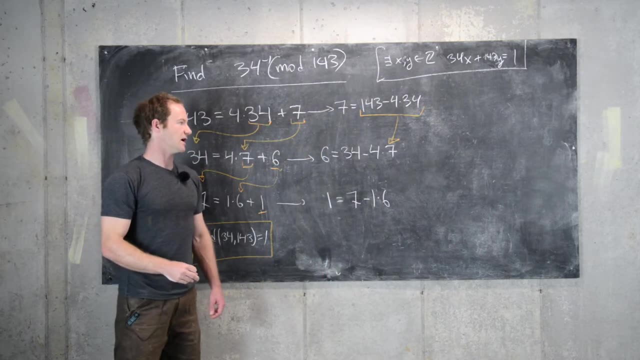 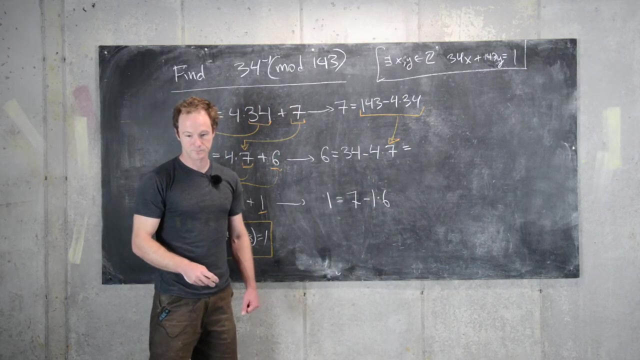 Good, And then, if you recall from previous videos, what we'll do is we'll take this expression for 7 and plug it into the value of 7 in the bottom equation, And what we'll see that we get here is the following: 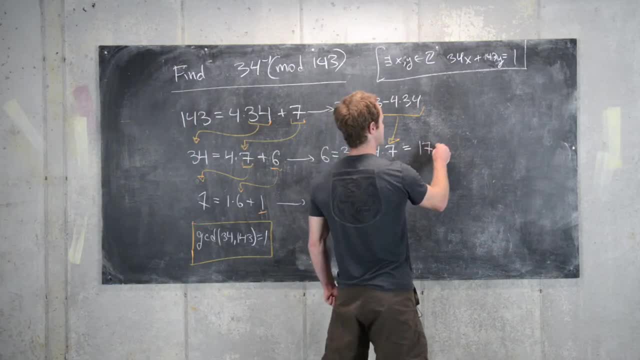 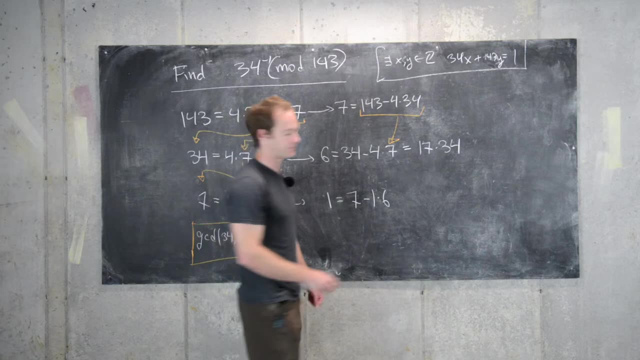 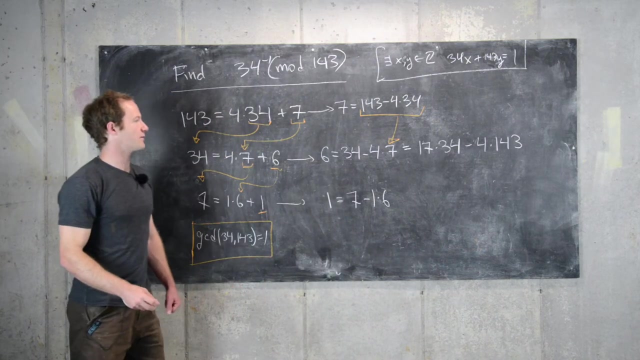 17 times 34.. So this is 17 times 34, minus 4 times 143.. So minus 4 times 143.. So that's what we end up with when we do that. Great, And now the next thing that we'll do: 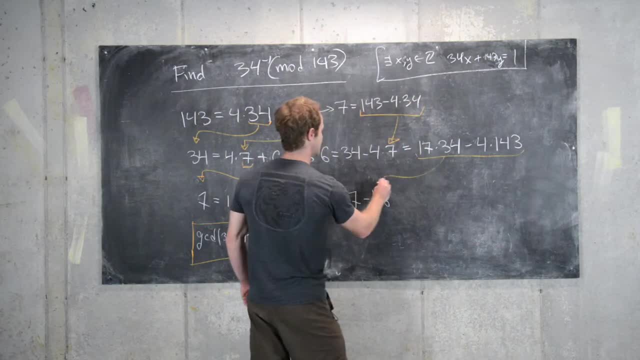 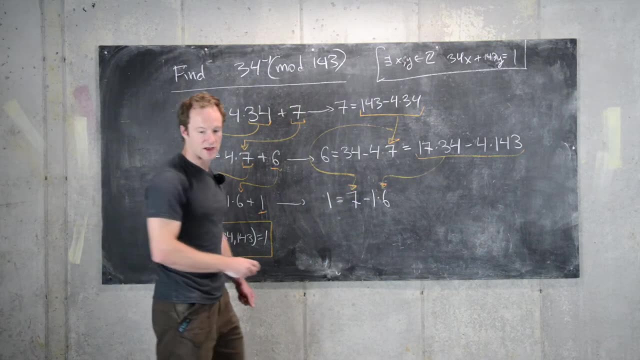 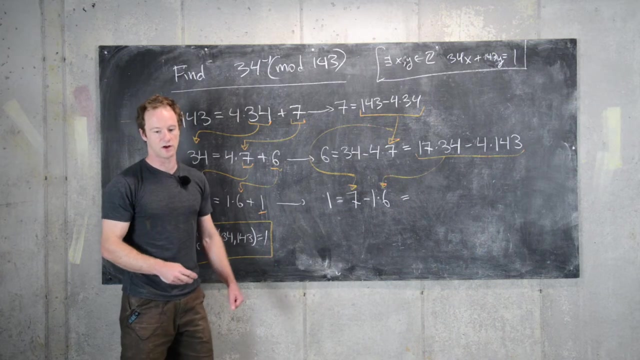 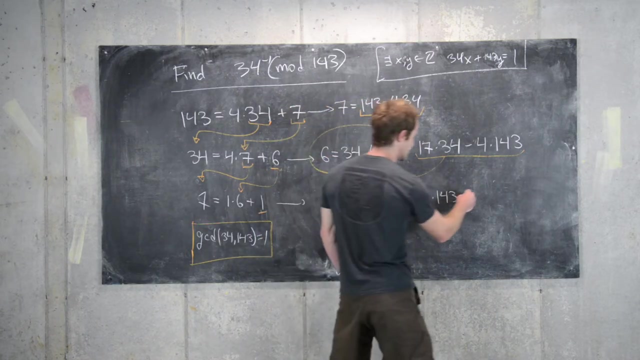 is: take this number for 6 and this expression for 7 and plug it in below And we'll end up with 1 equals. so I'm skipping lots of arithmetic here, but again, look at another video if you want that. So this is 5 times 143 minus 21 times 34.. 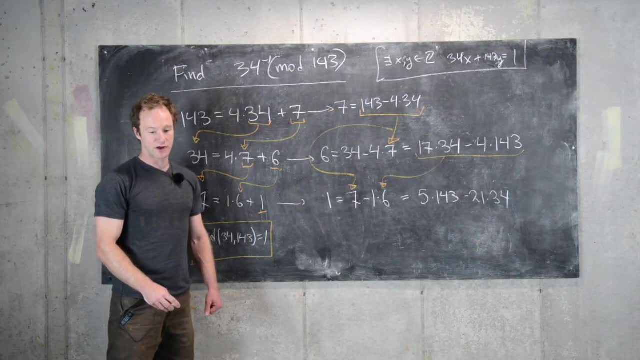 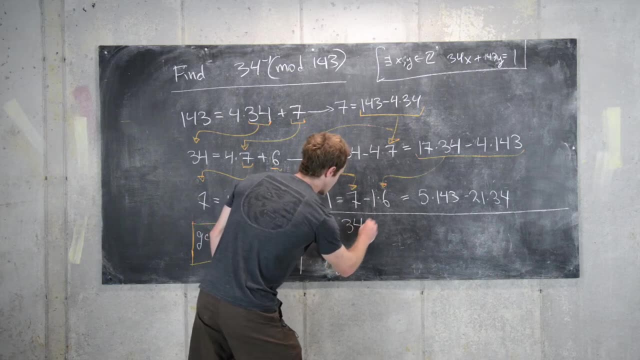 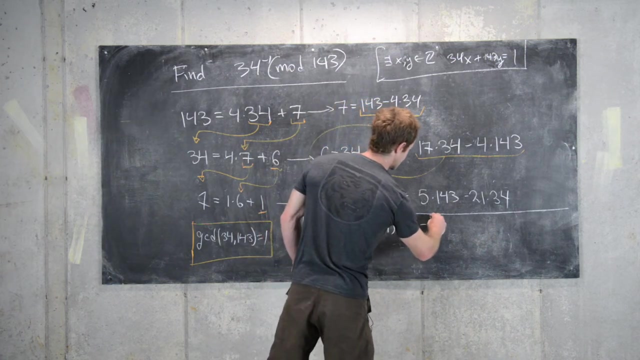 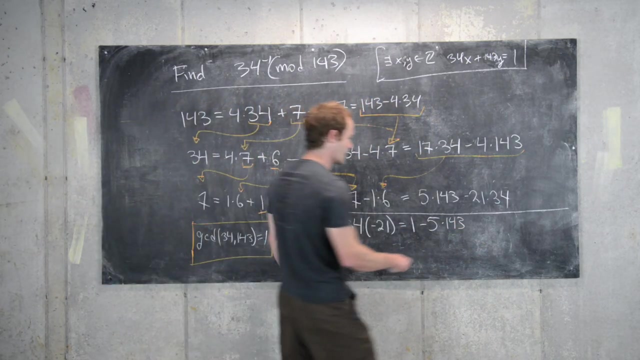 Good, And now what we can do is rewrite that as follows. We can rewrite: 34 times negative: 21 is equal to 1 minus 5 times 143.. Good, And now notice that number is obviously congruent to 1 modulo 143. 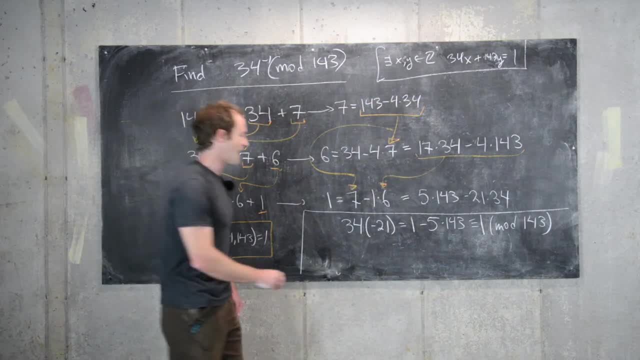 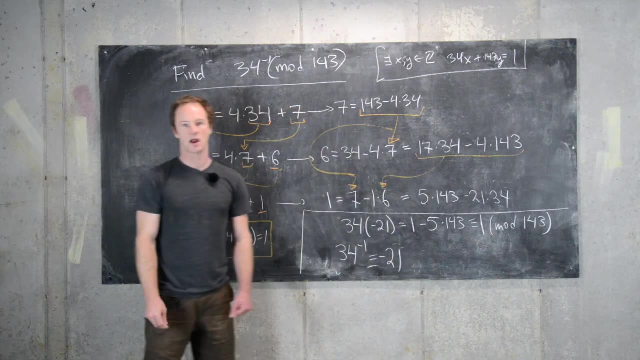 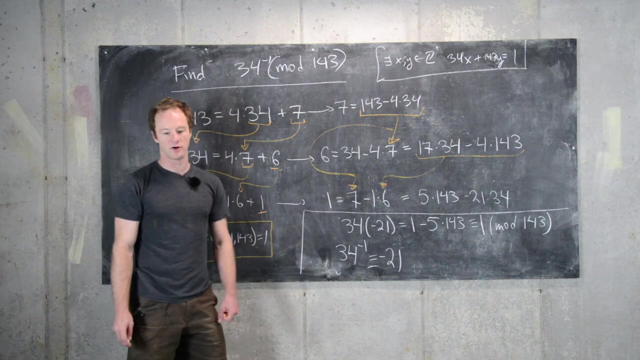 Good, And that tells us that 34 inverse is equal to negative 21 mod 143.. But we'd rather not work with negative numbers, so what we can do is just add a multiple of 143 to this, And what we'll end up with is: 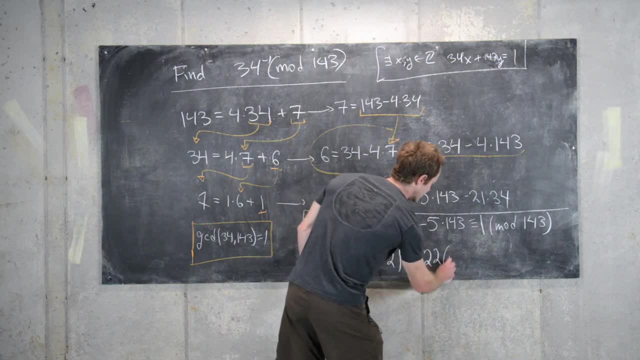 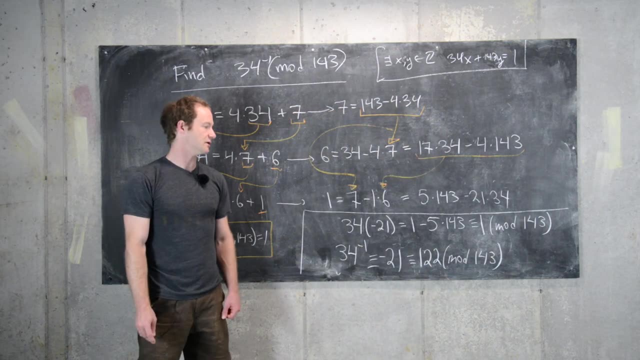 that this is congruent to 122 mod 143.. So 34 inverse. So 34 inverse is 122 mod 143.. Okay, That's the end of this example.